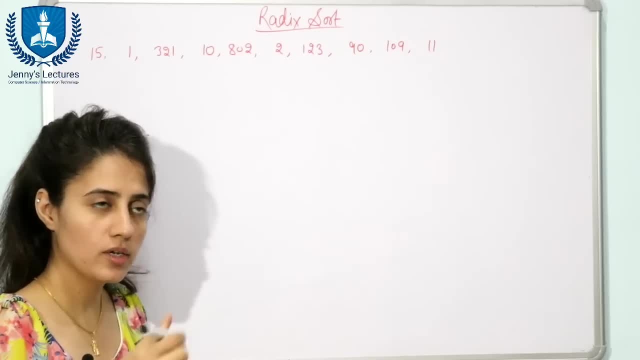 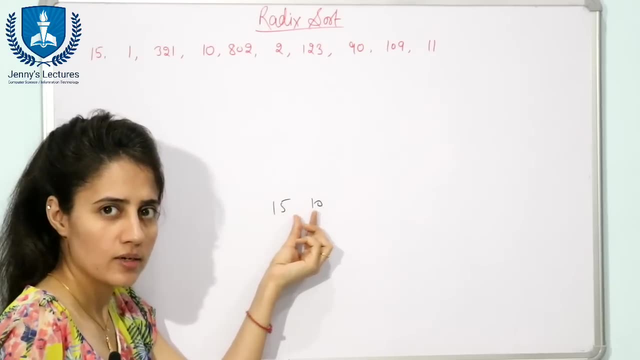 Here the numbers are not compared like this. see, we have done in another sorting algorithm, suppose I am taking 15 and 10, then I am going to compare this 15 with this 10. is 15 greater than 10? yes, then do swapping something like this. see, we are not going to do any comparison here between the 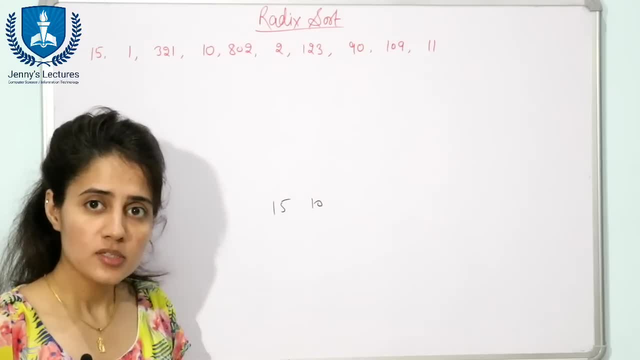 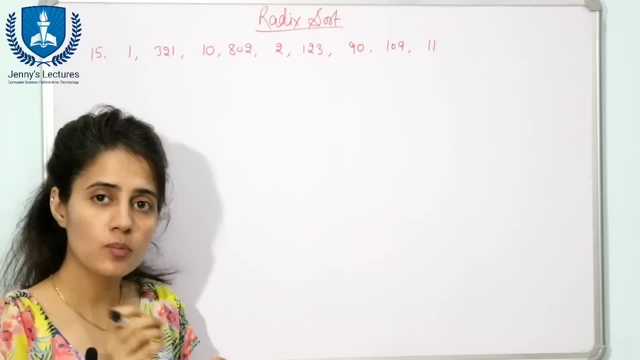 numbers given right. so now, if no comparison is there, then how the data is to be sorted? see. data is to be sorted here digit by digit. we are going to sort the data according to the place value of the digit, or you can say the position of the digit in that number: see. suppose we are. 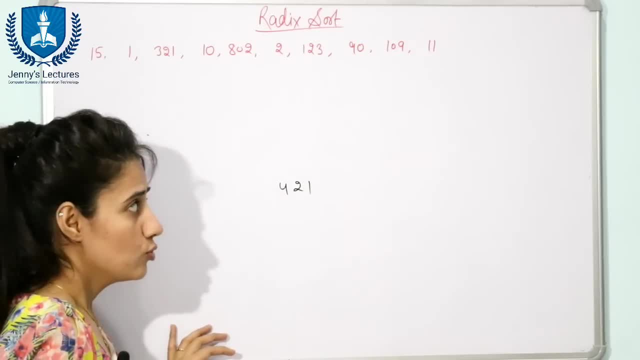 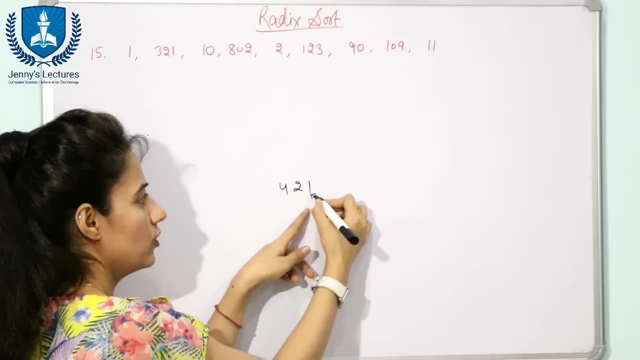 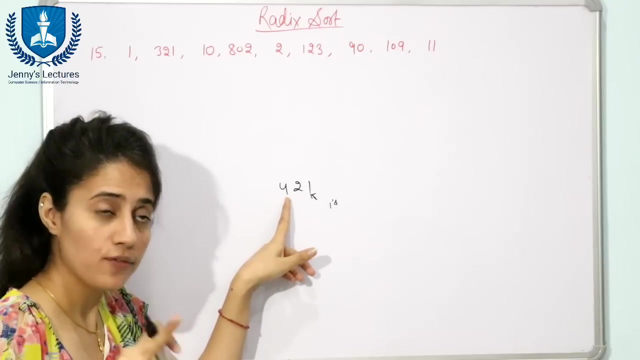 taking a number, 4 to 1, right. so this is what see. place value is what. here we have this. place value of this one is ones. place value of two is tens. place value of this four is hundreds. fine, and face value of this one is one. face value of this is two. face value of this is four. I hope you know. 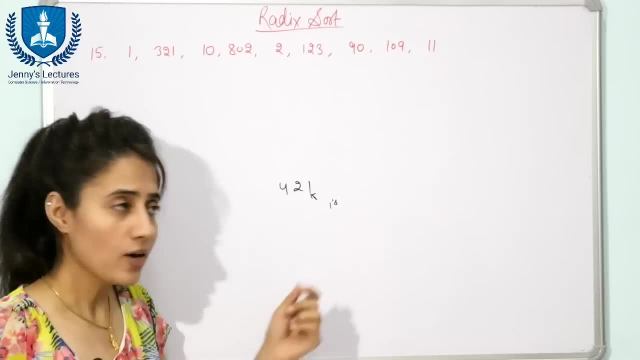 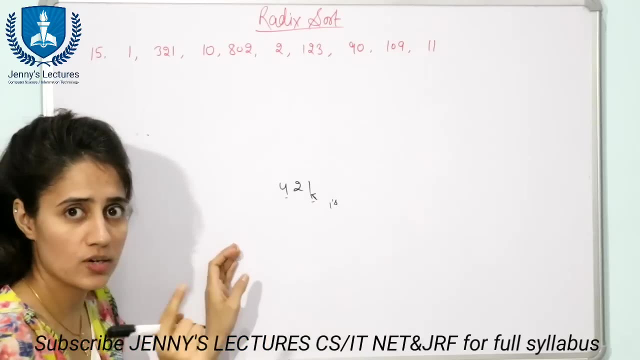 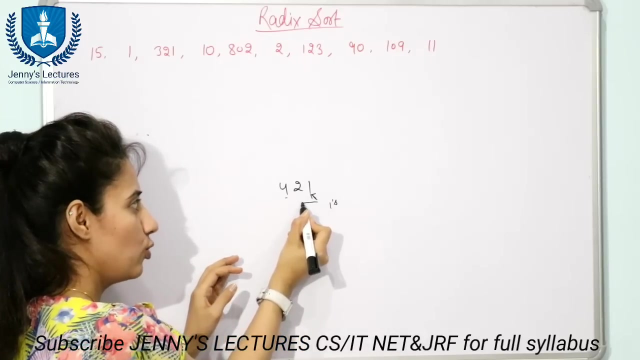 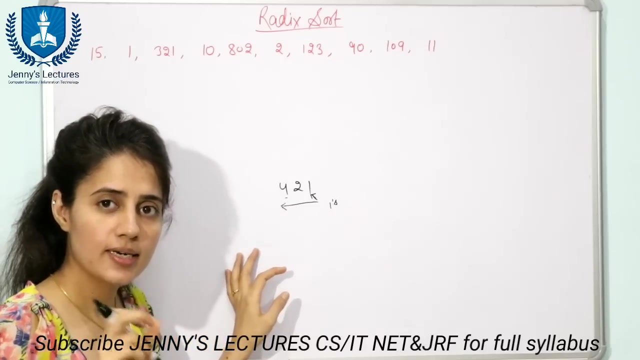 what is face value and place value right. So we are going to start from the least significant digit. least significant digit is this side and this is the most significant digit. So I am going to start this sorting from this least significant digit and we are going to move towards most significant digit right, digit by digit. the 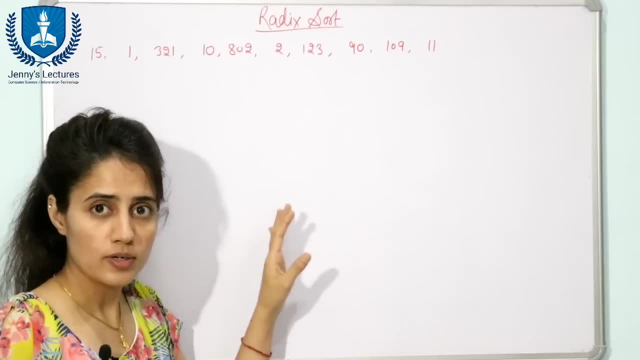 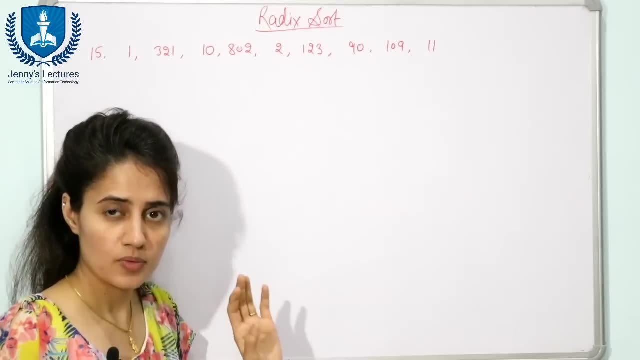 data is to be sorted. So see how the data is to be sorted, digit by digit. let us take this example. we are going to solve this one. we are going to solve this one. we are going to solve this one to. we are going to sort this data using reddick sort. fine, see the sorting algorithm we have. 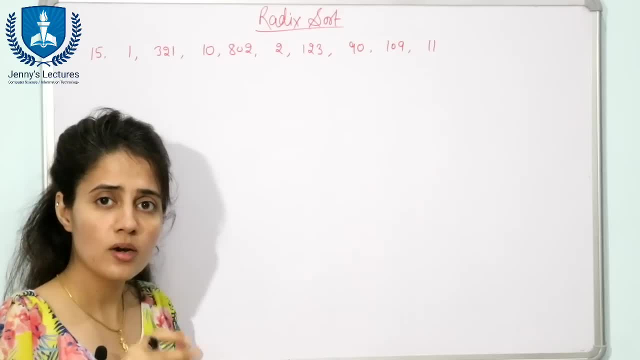 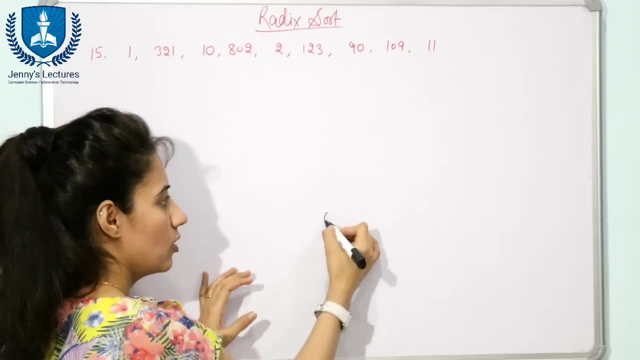 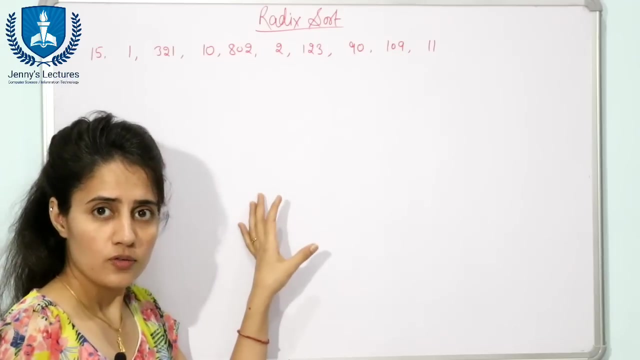 discussed bubble, quick merge, selection, insertion. those are comparison based sorting and the best, best time complexity for those comparison based algorithm is order of n log n, or you can say omega n log n. they cannot do better than this. so after sorting we are also going to see what is. 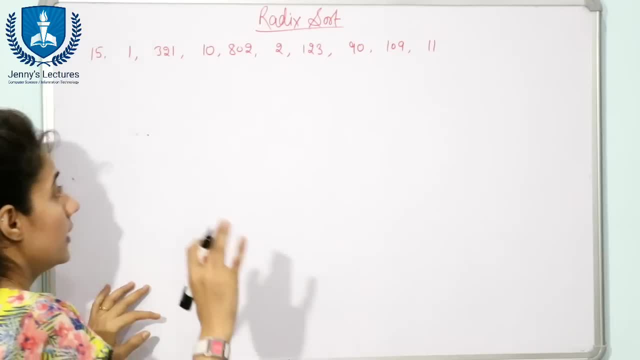 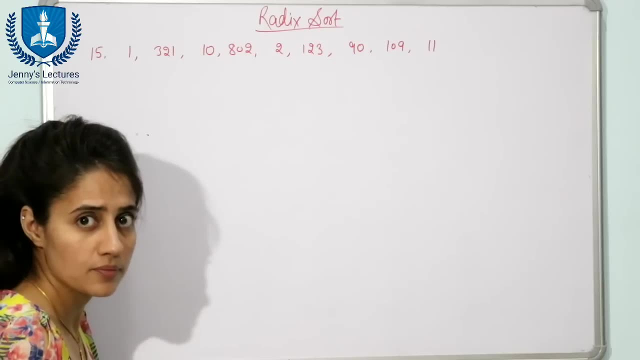 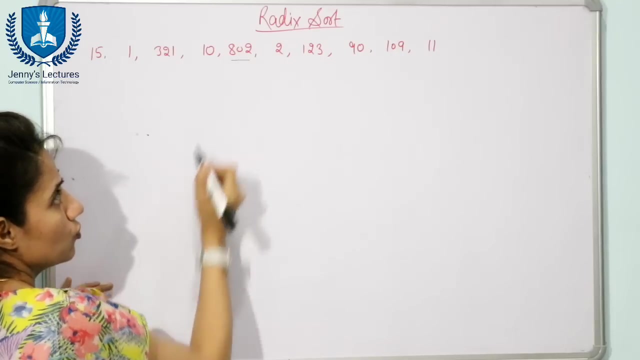 the time. complexity for this reddick sort? fine, see here. the first step in this sorting algorithm is: out of these given numbers, find out the maximum number. fine, now see. by looking at these number we can see the maximum number is what: 802. second step is calculate how many digits are there in. 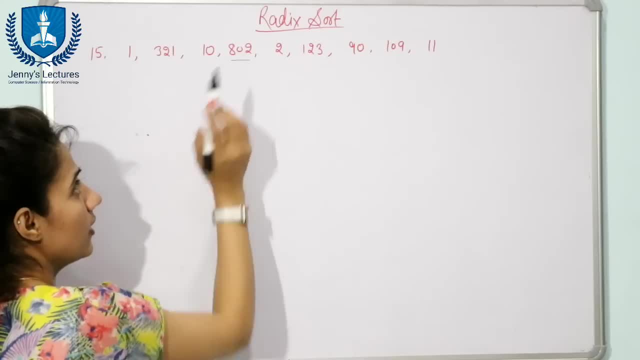 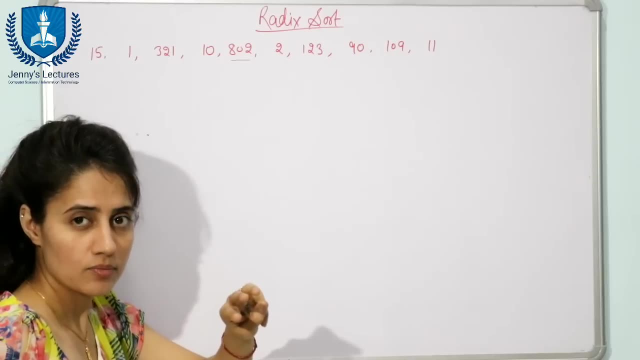 this maximum number? how many digits are there? one, two and three. now third step is you are going to calculate the time complexity for this reddick sort. fine, see here the first step in this number. we are going to make all these numbers a three digit number. right now, how we are going to. 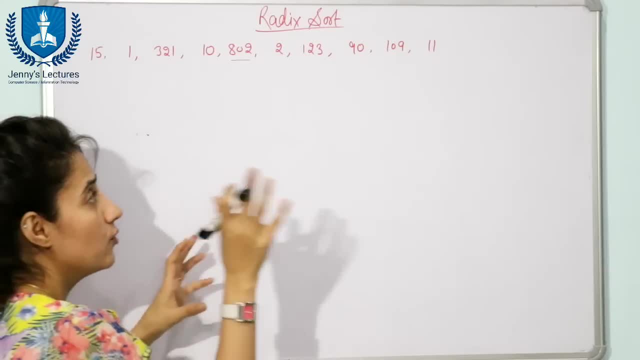 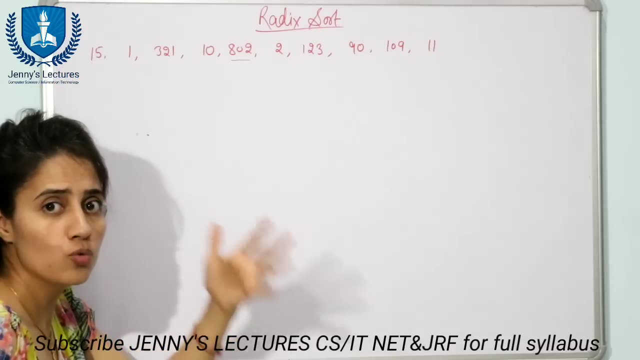 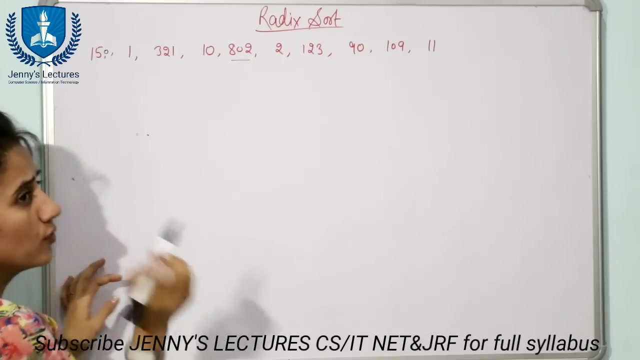 make you are going to put zeros. now where, where you are going to put zero, suppose this is the number. this is two digit number, one and two. now where you are going to put zero to make it a three digit number. you cannot put zero here, because if you put zero here then it will become 150 and the 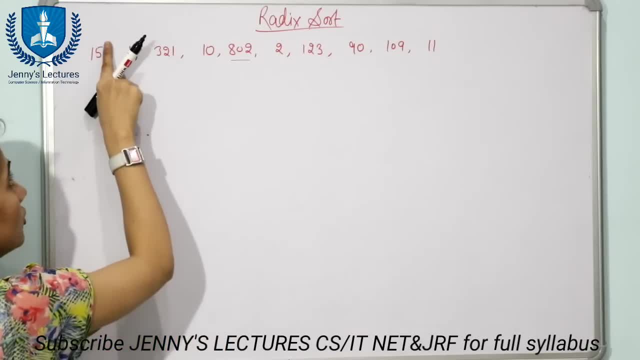 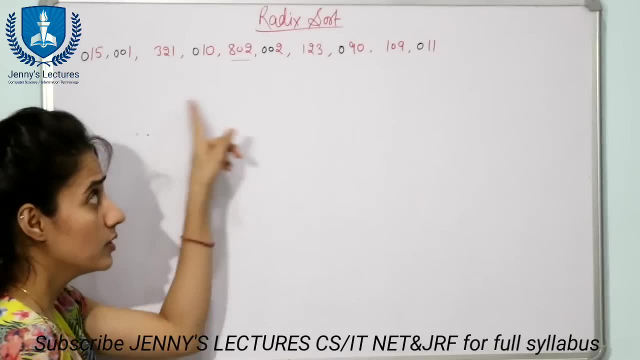 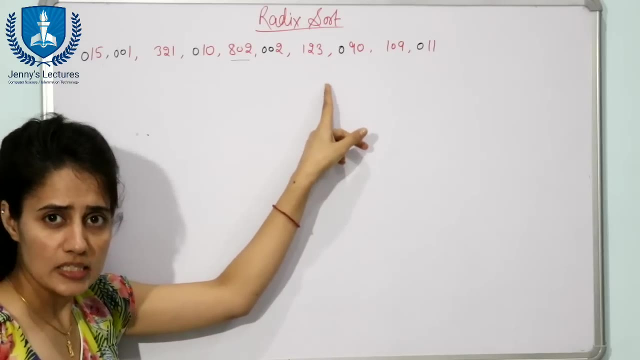 number is 15, fine, so you cannot change the number, the value of this number. that is why we are going to put zero to the here, this side. now all the numbers are three digit number, fine, red x means basically the base. so here i am dealing with decimal numbers. so base for. 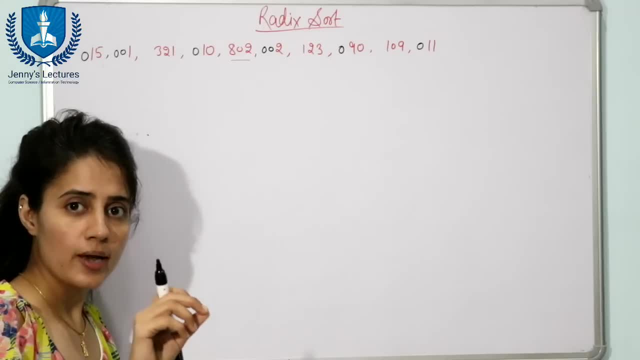 decimal number is 10, right? so that is why i am going to take 10 buckets. this is also known as bucket sorting. so here we are going to take 10, 10 buckets from 0 to 9. fine, see, this sorting algorithm is also used to sort. 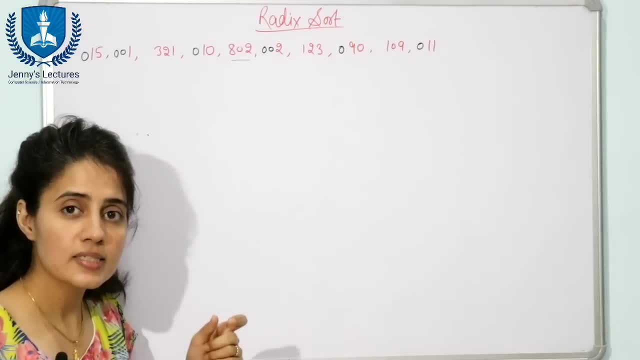 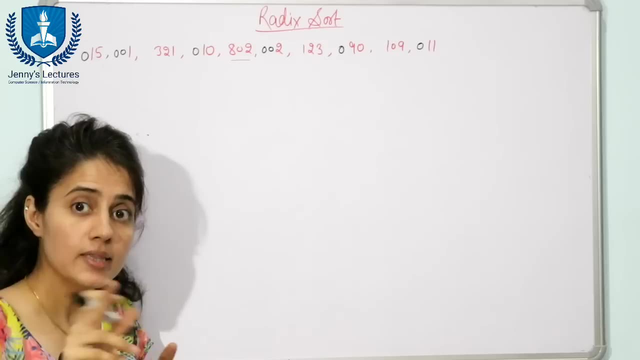 strings so you can say alphabets. in that case, the base is 26 for alphabets. so we are going to take buckets from 0 to 25, right? in that case, how we are going to sort? suppose i am going to take two names? 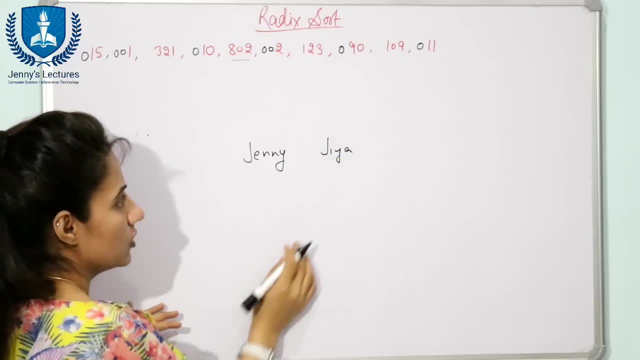 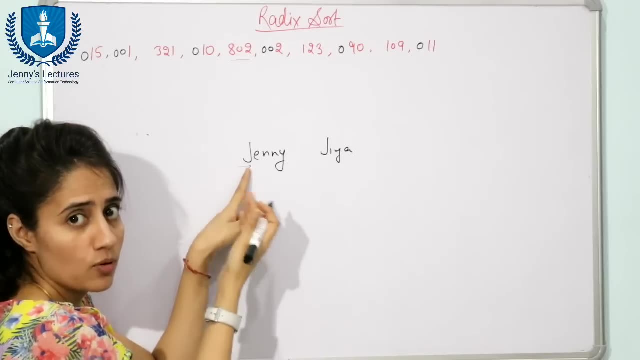 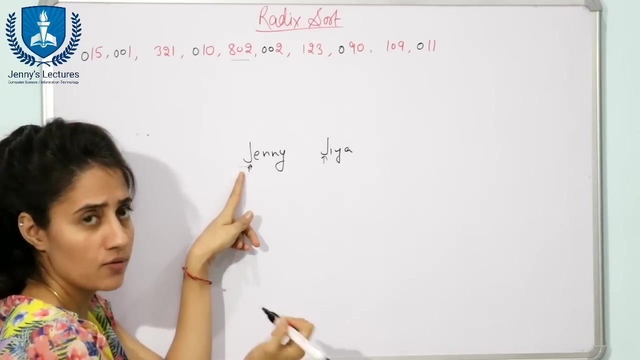 one is jenny and one is jia. so in that case we are going to start from here, or you can say from msb, you can say from the most significant bit, right? so we are compare with this, with this, both are j. then fine, again, we are going to compare. second, here we have here, we have i. so 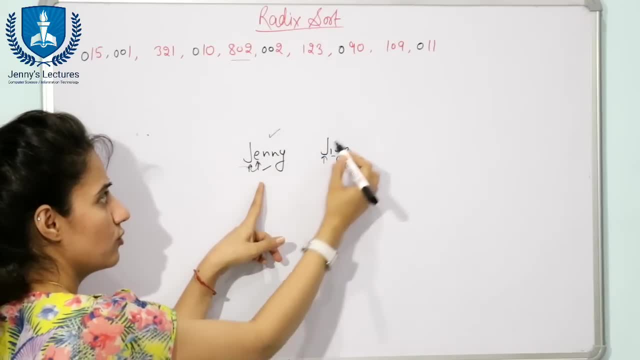 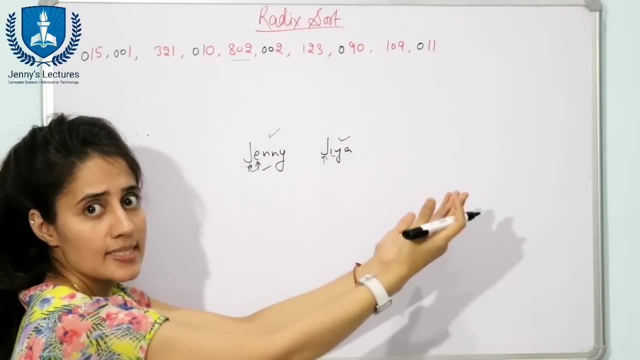 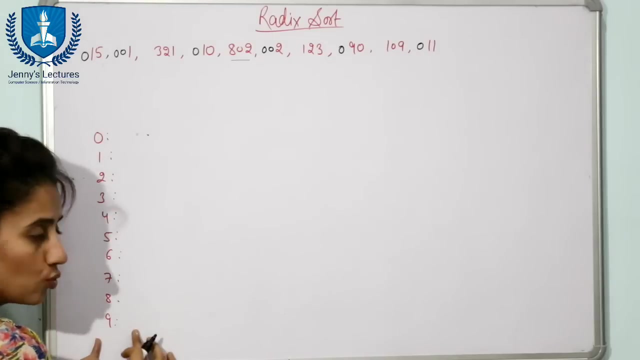 e comes first, then i. so this is this: jenny comes first, then jia. right, in case of numbers, we are going to, we are going to check from this side, from the least significant digit right now. see. so now we are going to take 10 buckets ranging from 0 to 9. right, and now we are going to put. 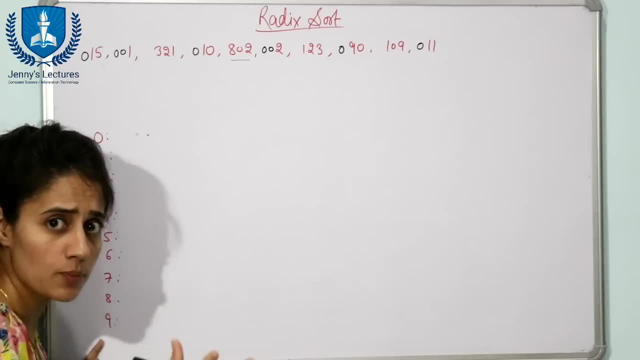 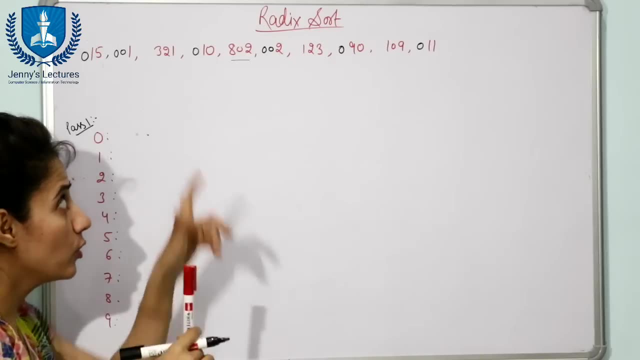 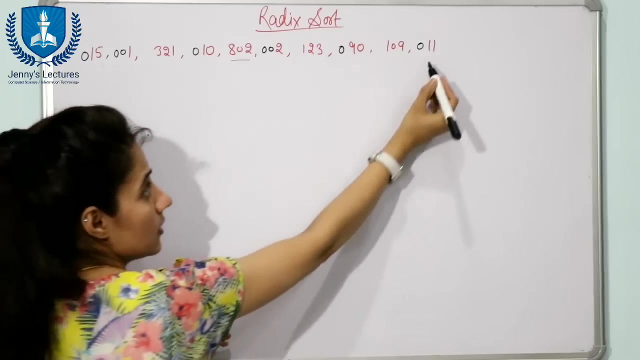 these numbers into these buckets. now the next step is how we are going to fill these buckets. see, this is pass one. so in pass one we are going to sort. we are going to sort these numbers according to which digit the least significant digit, and the least significant digit is this one. so we are going to check this digit of every number. 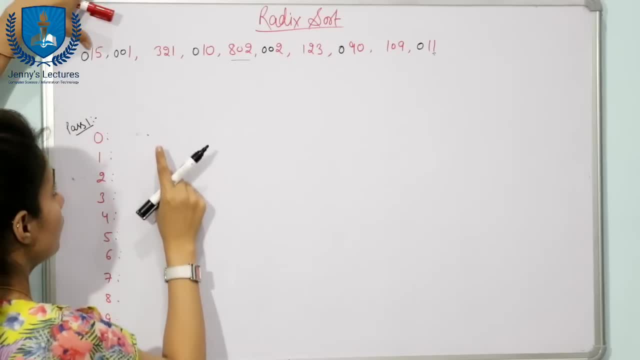 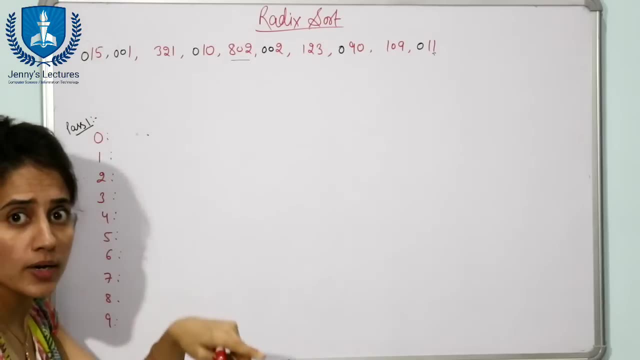 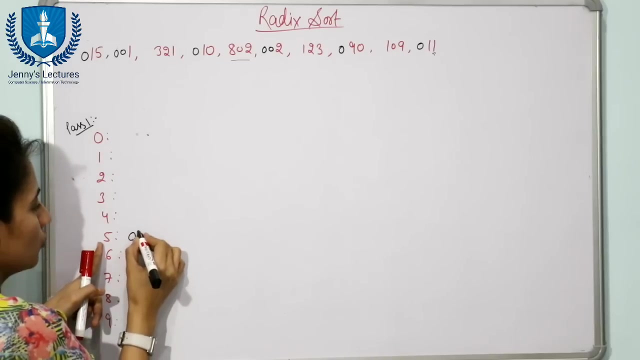 right and see. so first of all, check this number. the least significant digit is five. so now we are going to put this number in which bucket? in fifth bucket, the number, the bucket having number five. so here i am going to put this: one zero one, five. next number is zero zero one. now we are sorting. 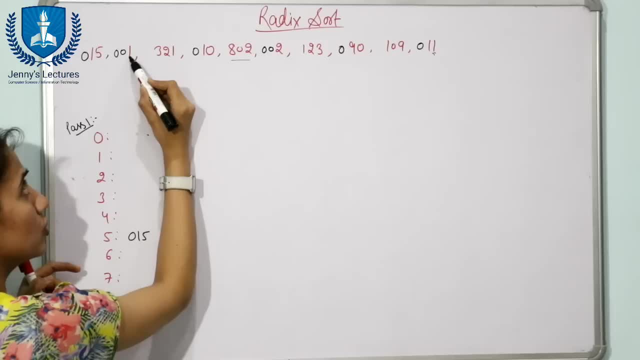 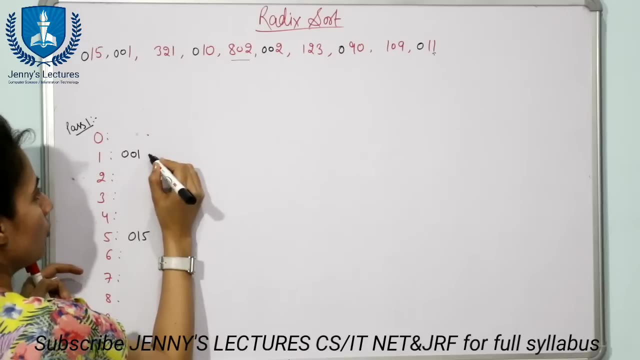 the data according to this, this digit, so i am just going to check this digit. here we have one, so i am going to put this in bucket one. here we have one, so i am going to put again this in one. here we have zero, so we are going to put this in zero. here we have two in bucket two. here we have two in bucket. 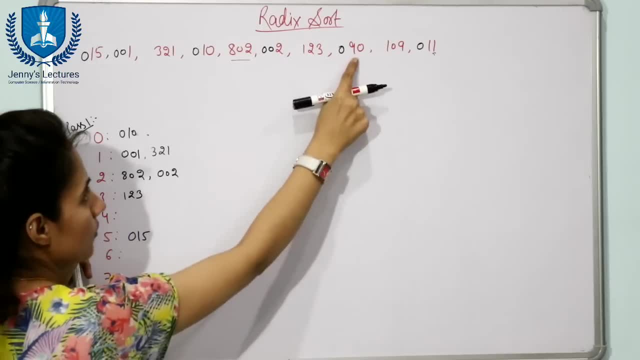 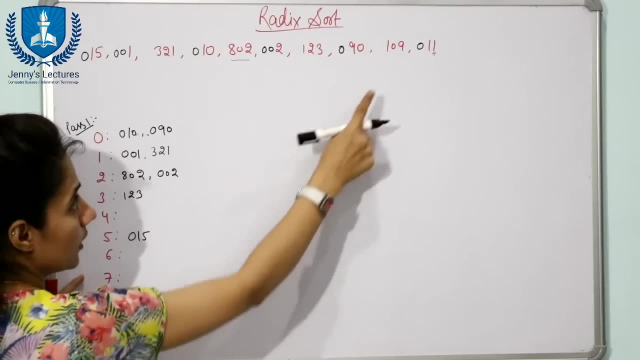 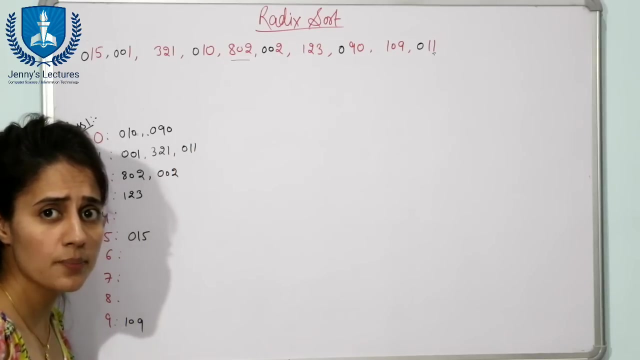 two: here we have three, so we are going to put this in bucket three. here we have zero. again, we are going to put this in bucket zero, then nine: we are going to put this in ninth bucket, and then one. we are going to put this in zero. one, one, one bucket right now. next step is you are going to remove the data from this. these: 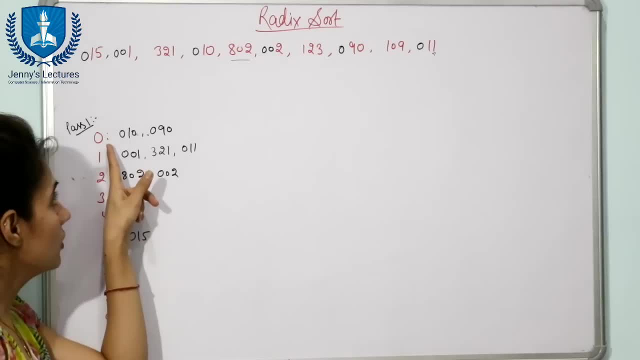 and how, starting from 0th bucket. now see, this bucket is having two numbers. now which number you are going to remove? first this number, the first number, right, not this number. you remember you are going to move this number first. so in 1th bucket also, from first this, then this, then 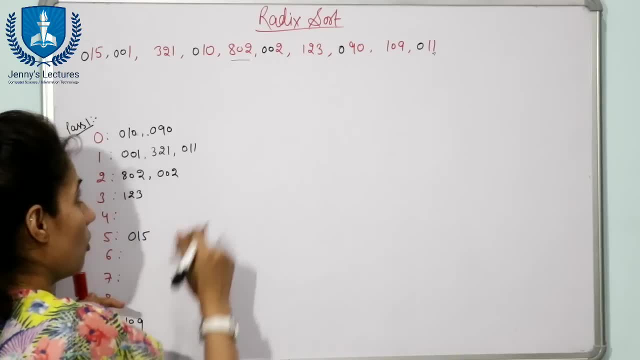 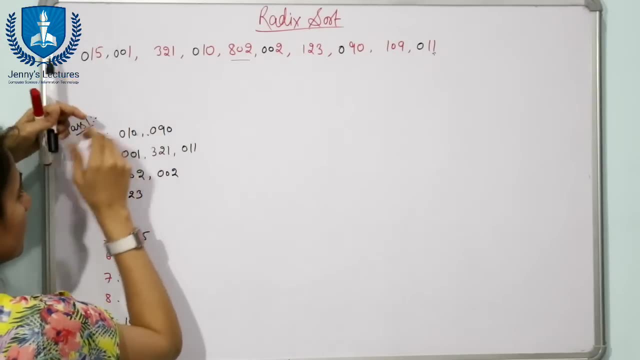 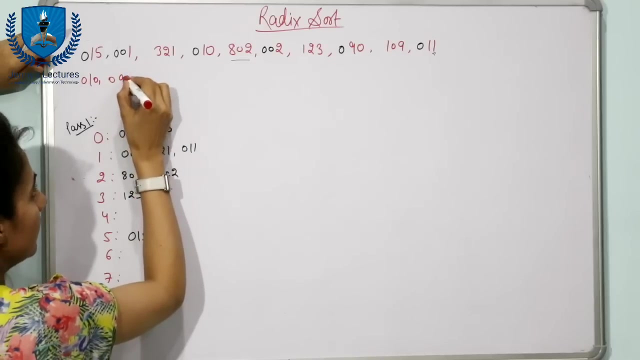 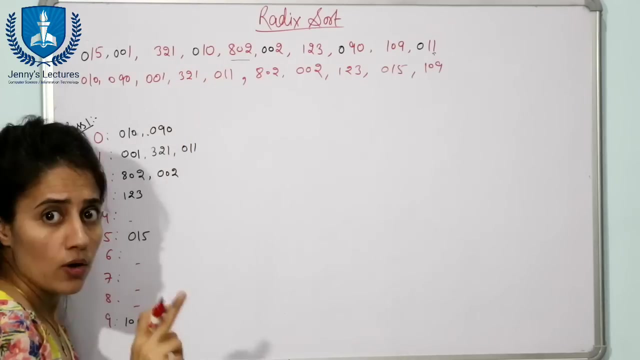 this now: remove one by one from data, from all buckets, and after pass one, after pass one, the data is something like this: first of all, remove this one, so the data is 0, 1, 0, then 90, then 0, 0, 1, then you remove 321, then 0, 1, 1. now, after first pass, the data is this one. so here one more thing. 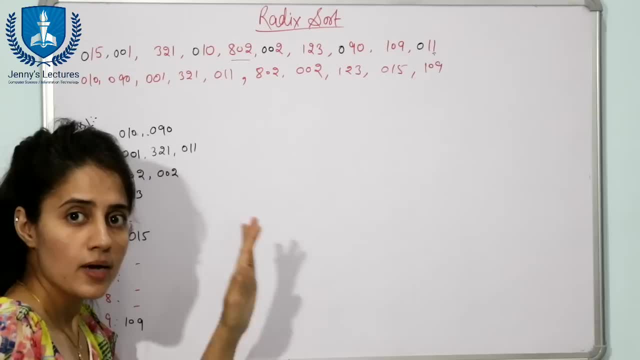 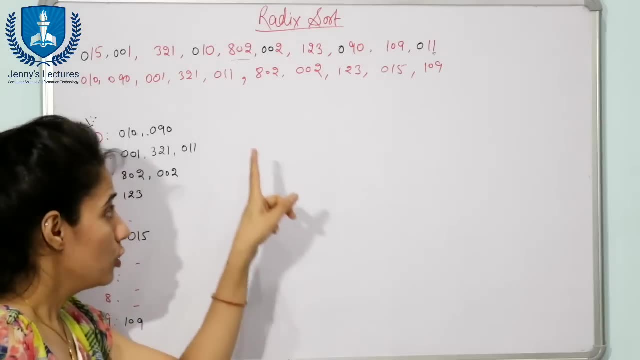 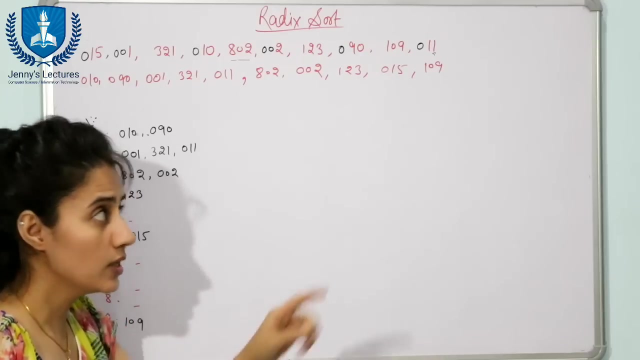 you have to take care. the passes would be same as number of digits in the maximum number. so maximum number is 802. number of digits are three. so here we have three passes. so after pass one, the data is something like this: now pass two. in pass two, we are going to sort the data according to which digit this. 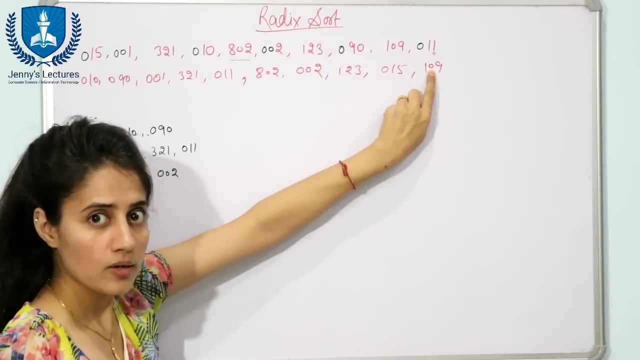 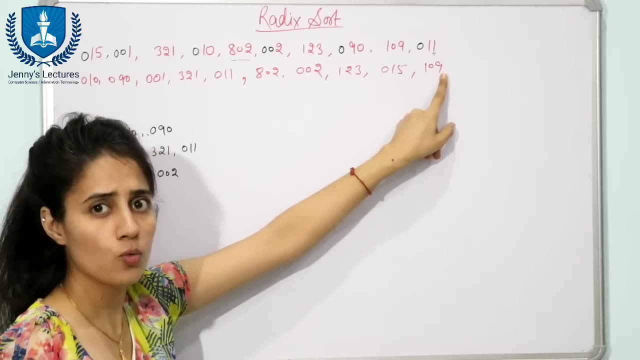 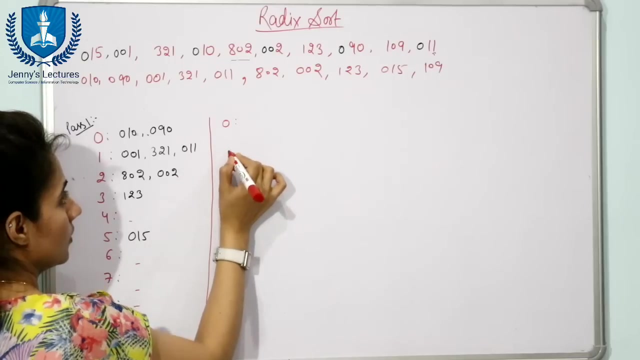 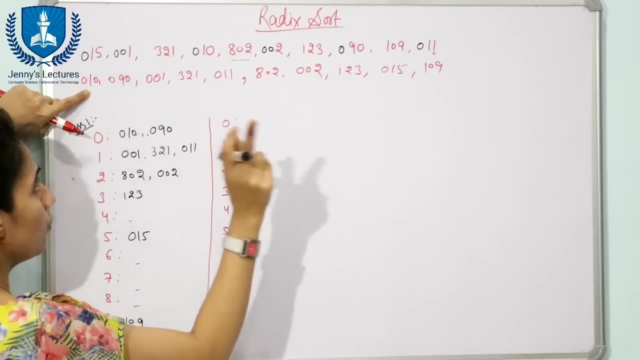 digit, the second one right, the digit which, which is at 10th place. we have already sorted the data according to this digit, the digit which is at 1th place right now. this digit, now again, we are going to take 10 buckets. now repeat the same step. check first number: this one: 0, 1, 0. now we are going to take which does it this? 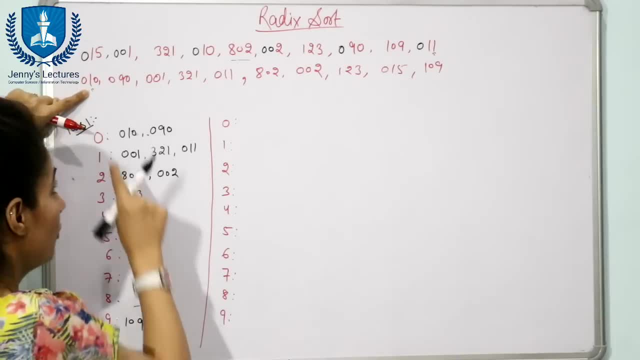 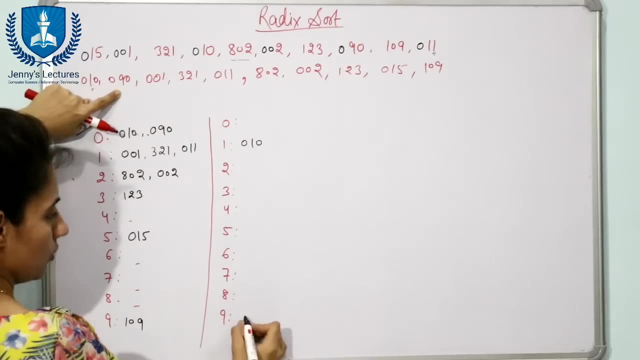 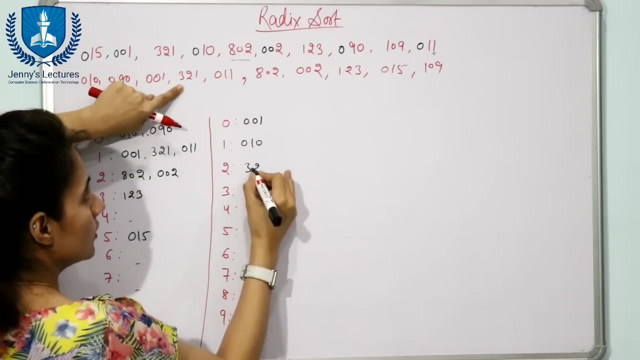 one, that is it which is at 10th place. now, here we have one, so we are going to put this in this bucket, bucket number one. we have nine, so we will. we are going to put this in this bucket. here we have 0: 0, 1 in 0th bucket 3: 2, 1, 2. second bucket: 0, 1. 1 in 1th bucket, bucket 802: 0 is there, so 802. 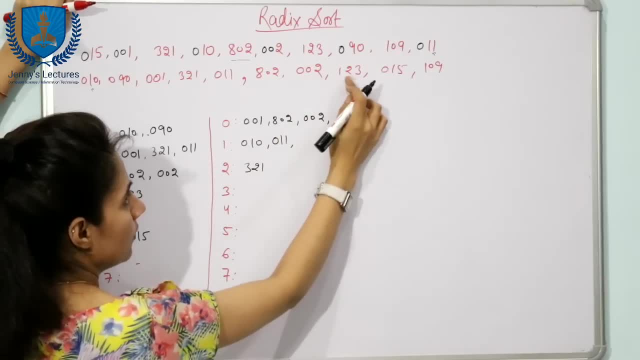 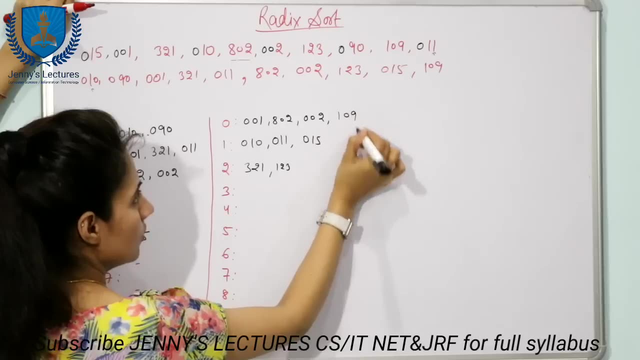 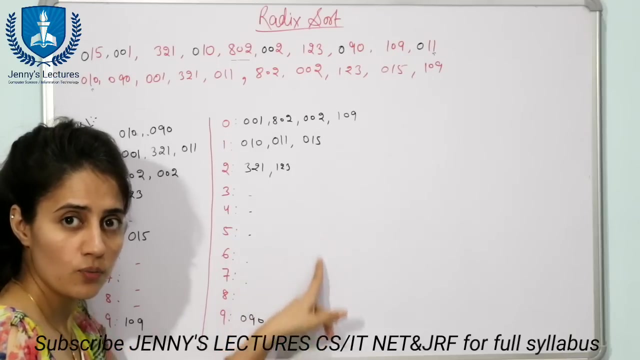 here also we have 0, here we have 2, 1, 2, 3, here we have 1 0, 1, 5, and here we have 0, 1 0, 9. these buckets are empty, fine, so that's fine. now next step is what? you are going to remove the data from these. 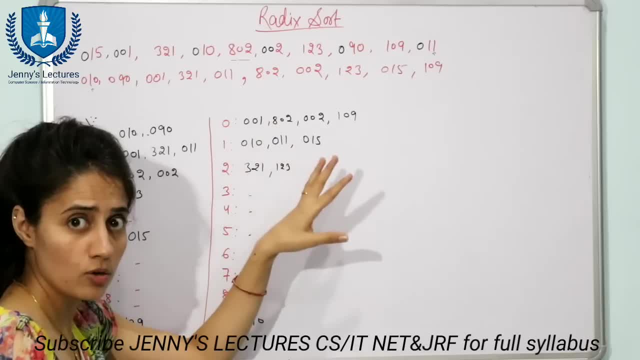 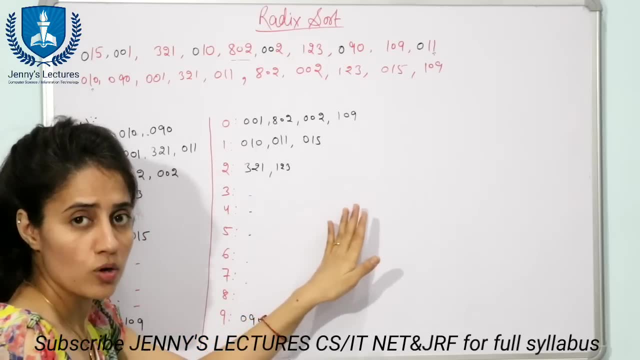 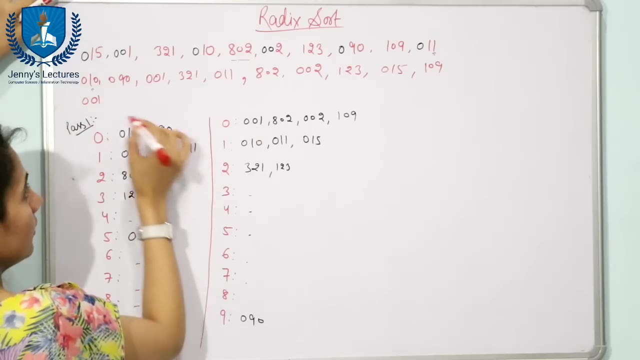 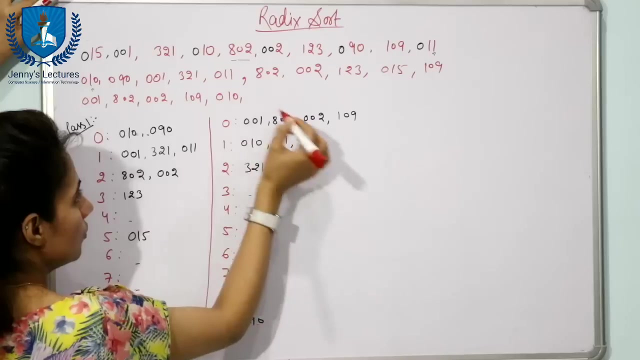 buckets and how: from the starting bucket and from starting bucket also, if many numbers are there, then we are going to remove the first number first, right. so after pass 2, this is pass 2. so after pass 2, the data is something like this: remove this one: 0, 0, 1, 8, 0, 2 0 0. 2. 1, 0, 9. here we have 0, 1, 0. so after pass 2, the data is: 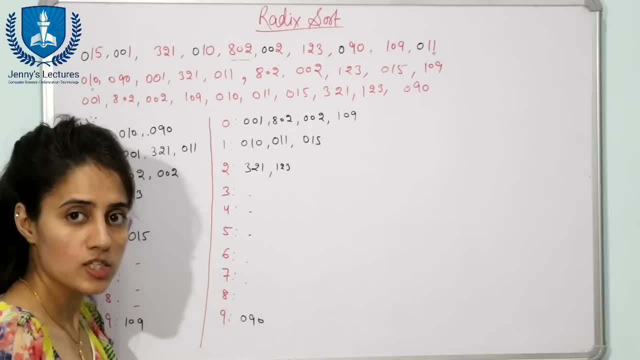 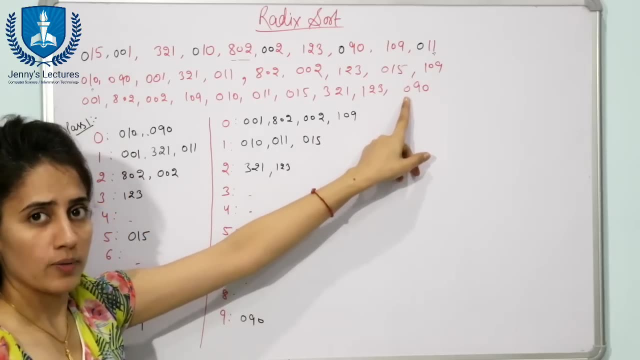 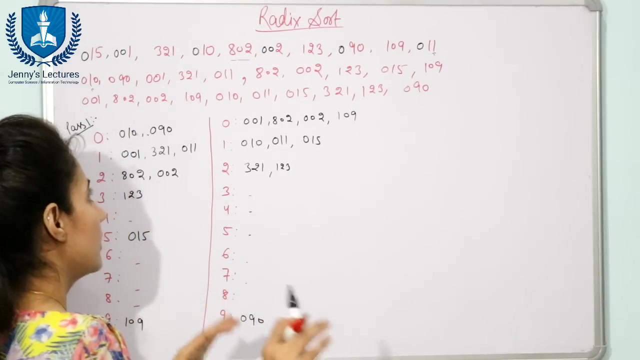 this one, now the last pass, that is the third pass. in that pass we are going to sort the data according to which digit? the third one, this one, the digit which is at 100th place right. so now say: repeat the same step. we are going to take again 10 buckets. now. this is pass 3. again, we are going 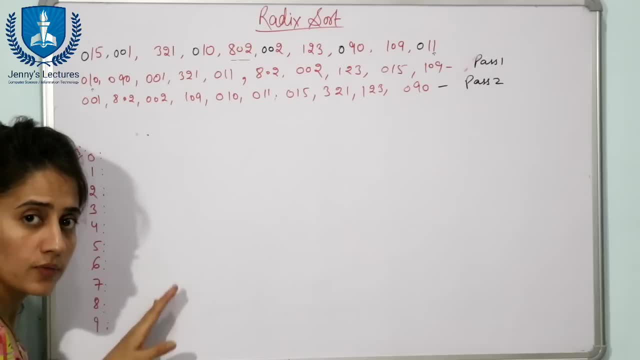 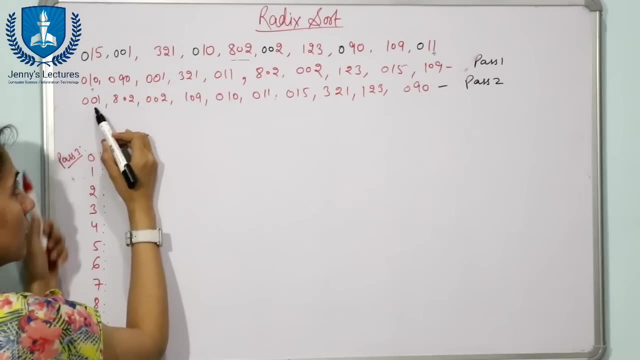 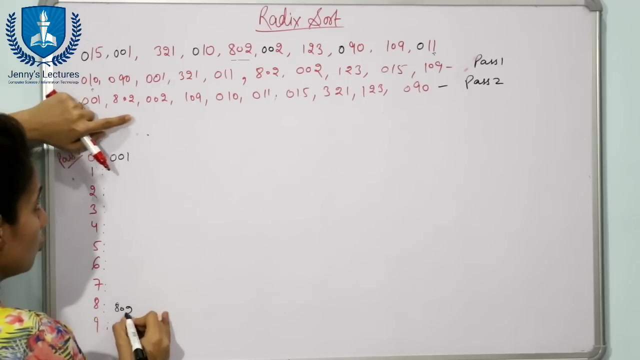 to take 10 buckets ranging from 0 to 9. again, we are going to fill these buckets. how so? these are the number after pass 2. so now we are going to see which digit, the third, one, third one. so now, here we have 0. we are going to put this in 0th bucket. here we have 8 802 0 002 109. 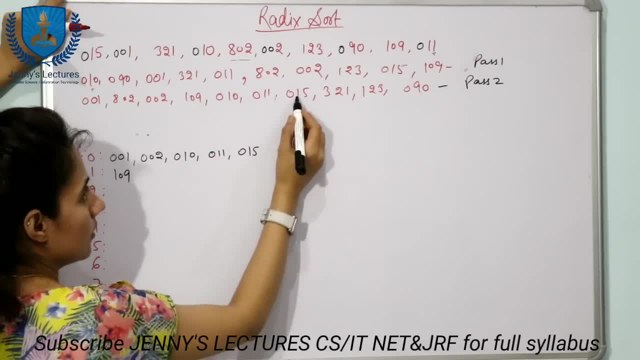 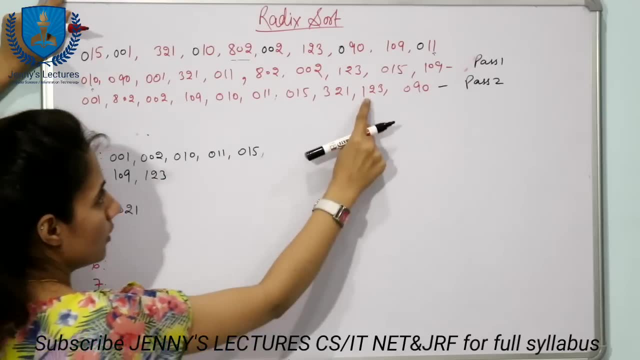 0, 1, 0. here we have again 0, 1, 1, 0, 1, 5, 3, 2, 1, 3, 2, 1, 1, 2, 3, so digit is 1. here we have 0, 0, 9, 0, right, so these: 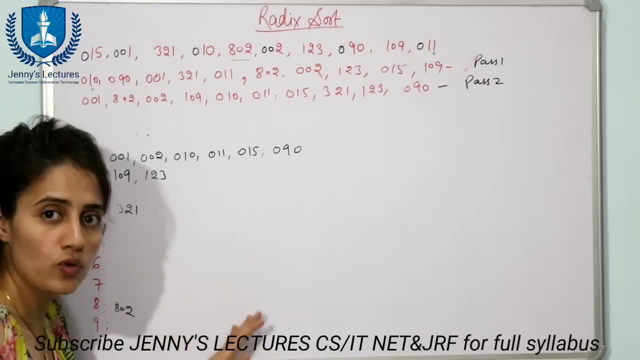 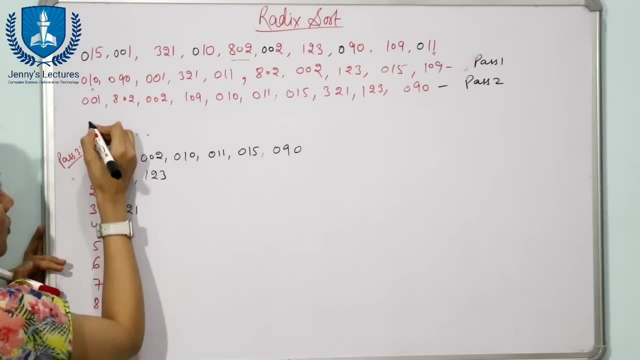 are the buckets now. now next step is what? you are going to remove data from these buckets. right, and remove means we are going to store the data in an output array. so here is 0, 0, 1, so you can write. 1- here we have. 2, here we have. 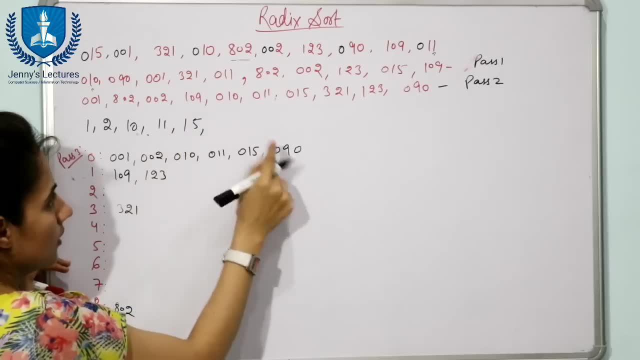 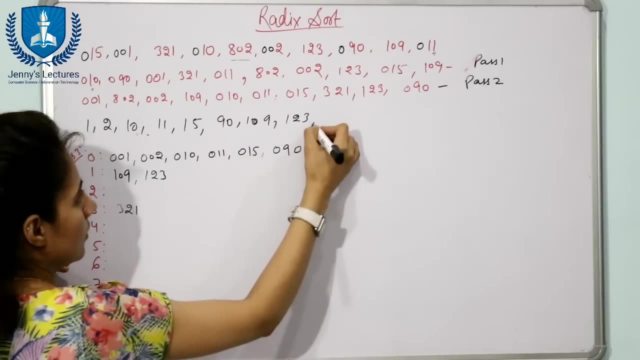 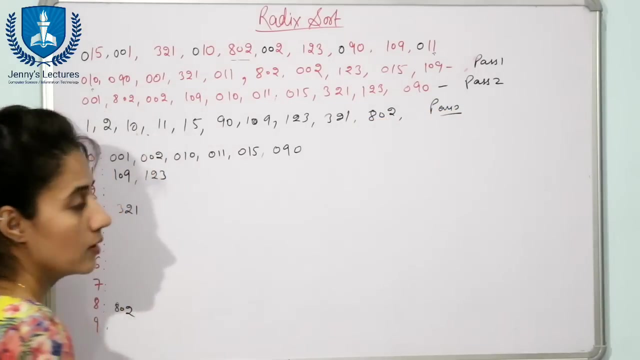 10, 11, 15, 90, 1, 0, 9, 1, 2, 3, 3, 2, 1 and finally 802. so this is the data after pass 3. so, as you can see, this is the sorted data now. so here we have removed the extra zeros we have put to make. 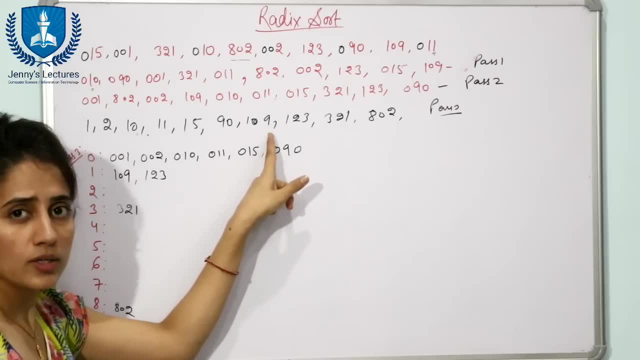 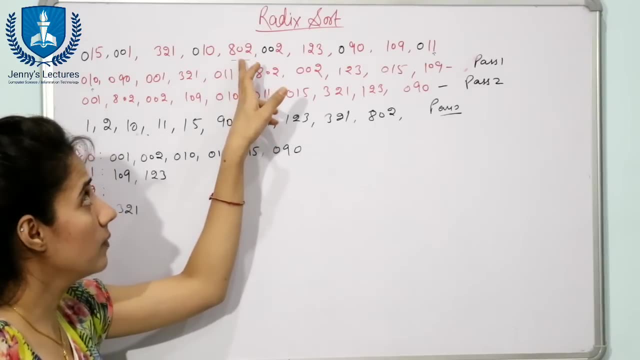 the numbers: 3 digit number right. so this is now the sorted data, as you can see how many passes are required. 3 means the number of digits. in the maximum number those number of passes would be required. here we have 3 digits, so 3 passes would. 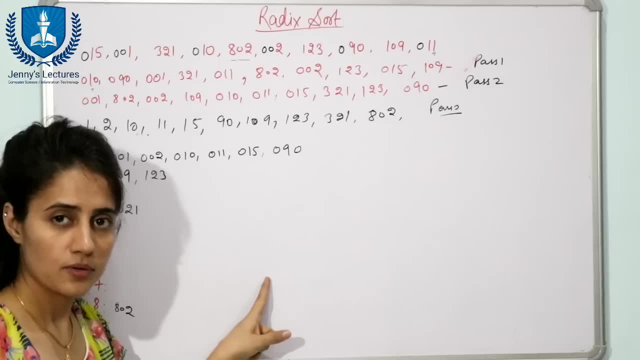 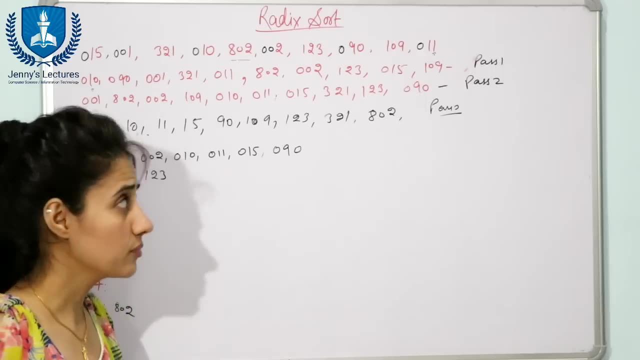 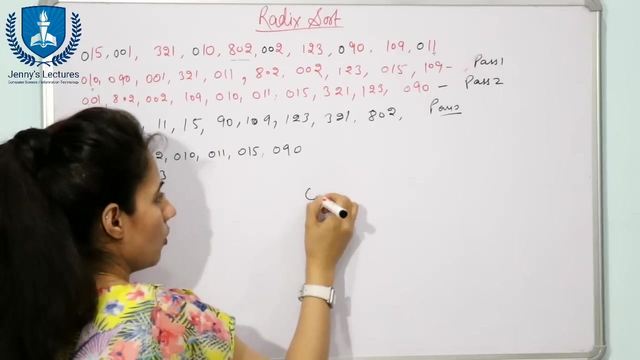 be required. so this is how reddick sort will sort the data. see this: reddick sort use what count sort as a subroutine. so you know what is the count sort, right, and if you say the, the running time complexity for this sort is what you can write order of. 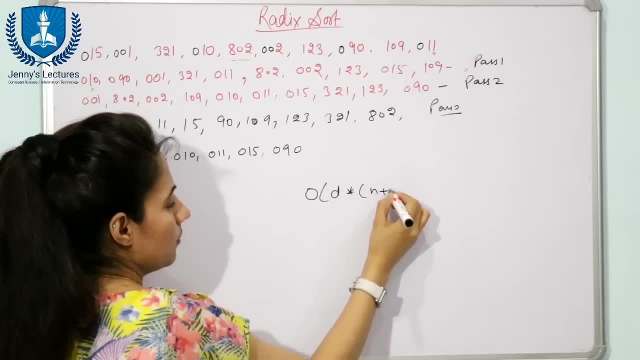 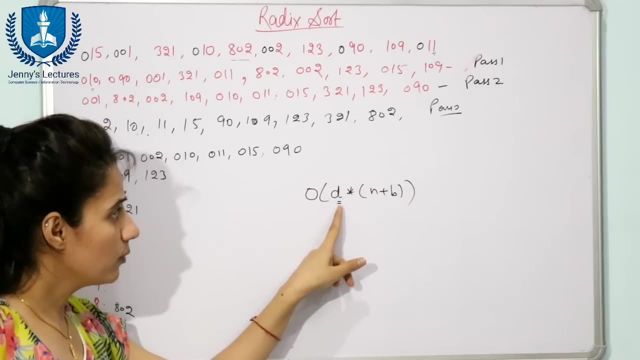 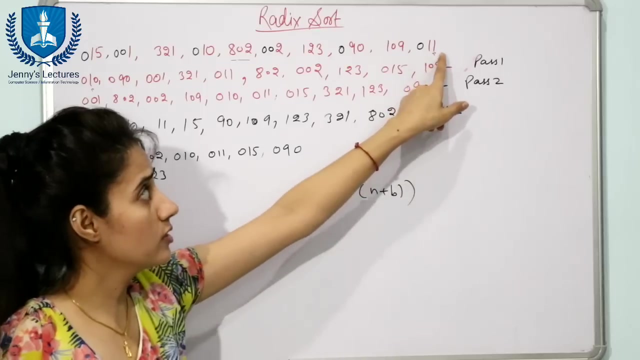 d into n plus b. now here see, d is what number of digits in maximum number. number of digit are 3. so here for each digit, we are going to repeat the steps right, first of all for this digit, thenbit, then this: how many times? 3 times we have repeated. so here we are taking d into n is the numberouring.